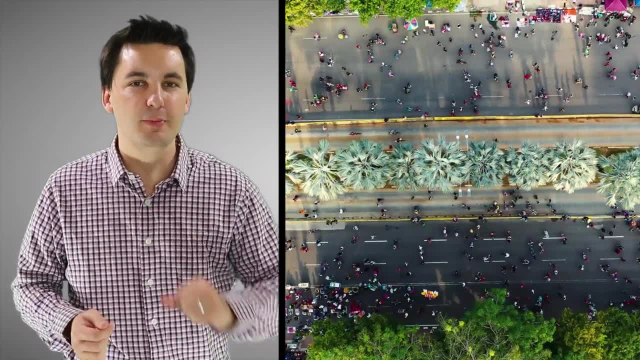 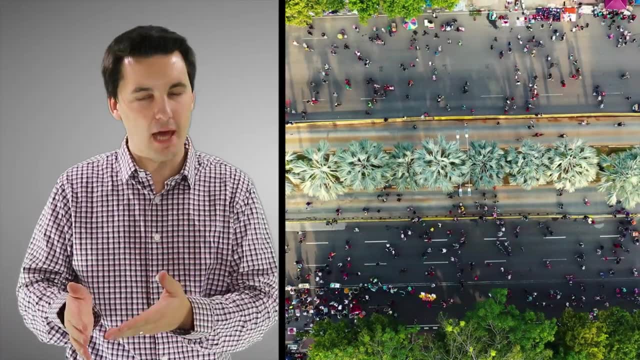 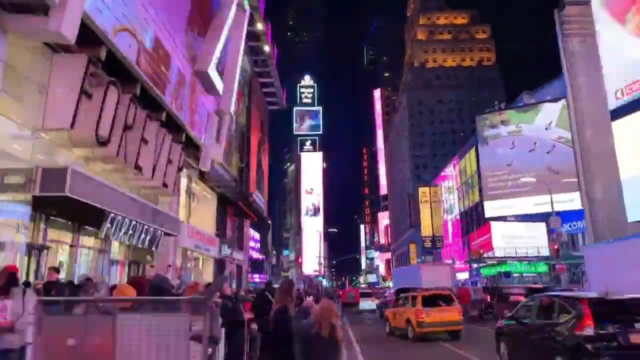 Think about the emotions that a place holds, Those physical components, those human characteristics. they help us create a sense of place in our mind. These feelings are based on experiences that we have with a particular geographic location. For example, if you go to New York City and you're walking down Times Square, you can feel right away a unique sense of place. 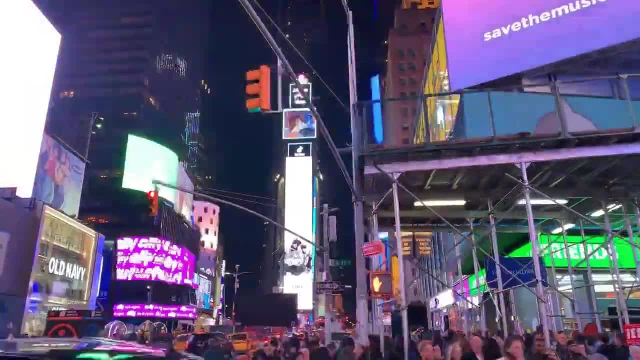 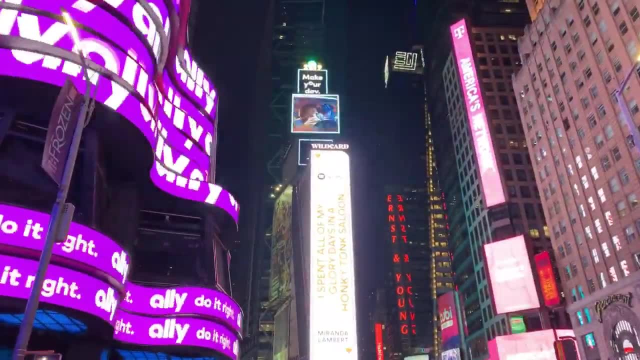 You can pick up on the sense of the fast-paced society, the bustling and the hustling of the streets, the economy that's thriving- All these different aspects make a unique sense of place for New York City. New York City is full of cultural and social expressions. 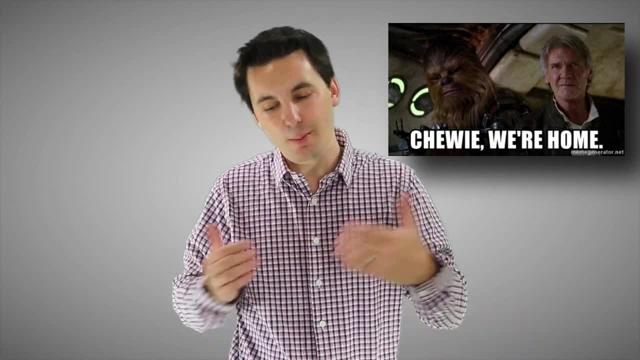 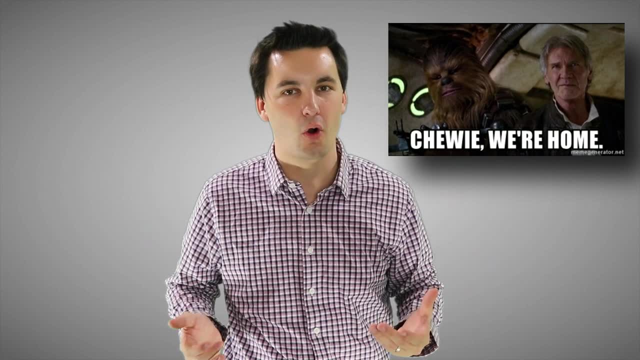 city, or if you've been on vacation for a long time and you come home- or maybe you've been away at college- that first time you re-enter your city or your hometown, you can just feel like you're at home. these things give us a unique sense of place and they're all defined by the different physical 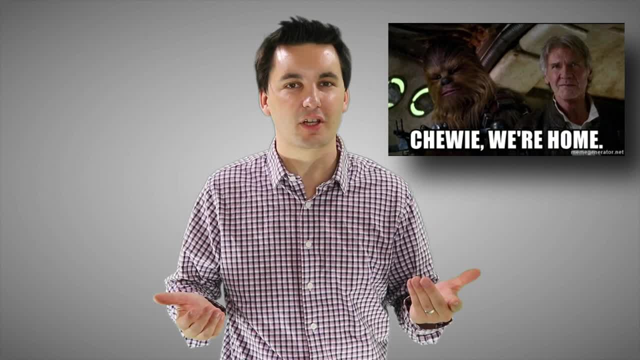 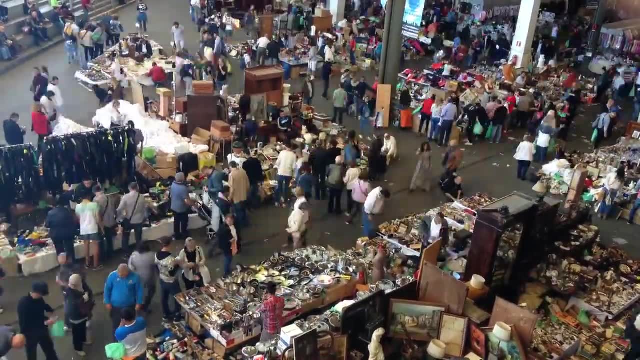 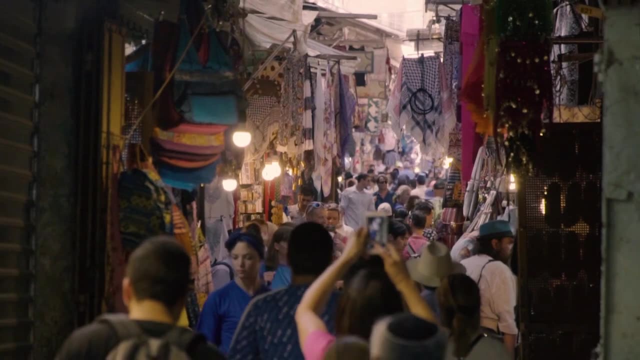 features we see, but also those humanistic characteristics that we become so accustomed to. we can gain this sense of place by looking at the different uses of public spaces, how people are interacting, how the physical terrain has been shaped, all these different things, all the way to the ethnic breakdown or the religious components. the languages that are spoken help identify in. 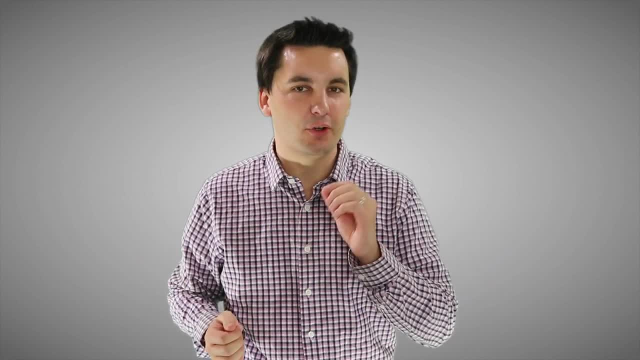 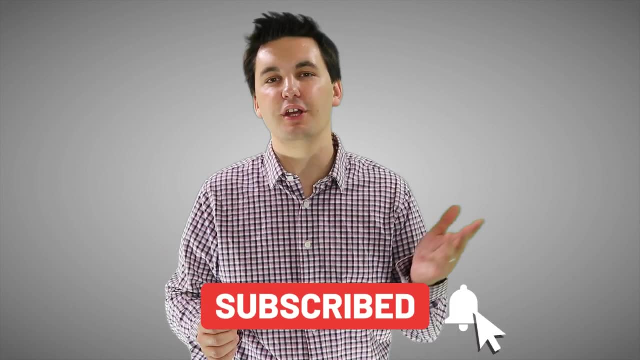 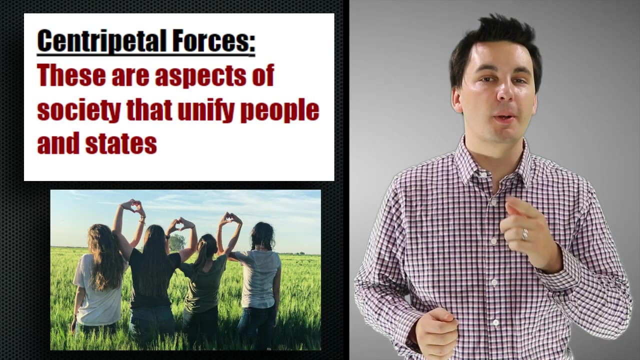 our minds that sense of place. now, when looking at places, we can also see different centripetal and centrifugal forces at work. these are defined by different languages, cultures, ethnicities, religions, attitudes and beliefs, governments. all these things both help hold the society together and also push people apart. centripetal forces are forces that pull people. 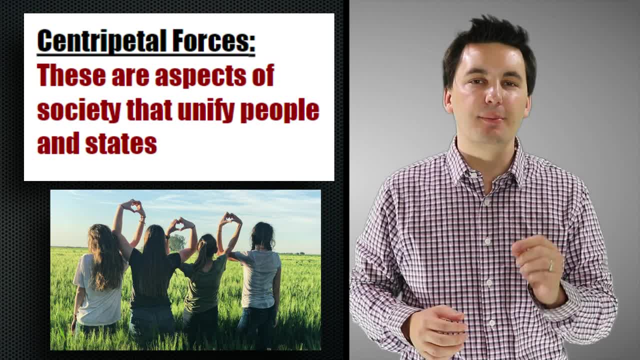 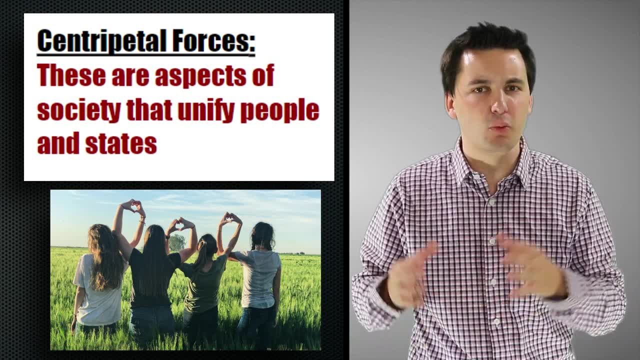 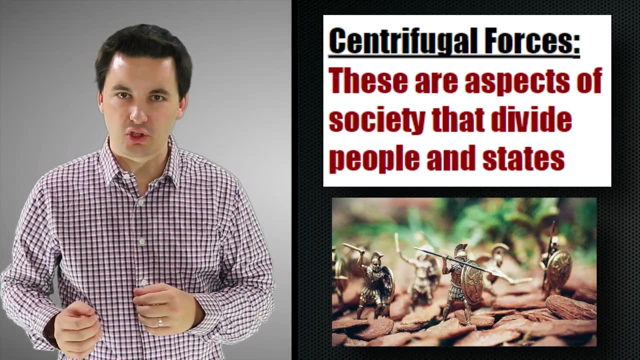 together. they hold the society as one. oftentimes this can be because of a common language that's spoken, a national identity, a homogenous community. all these things would make a united identity for a place and they pull people together. on the other hand, societies that have multiple languages, 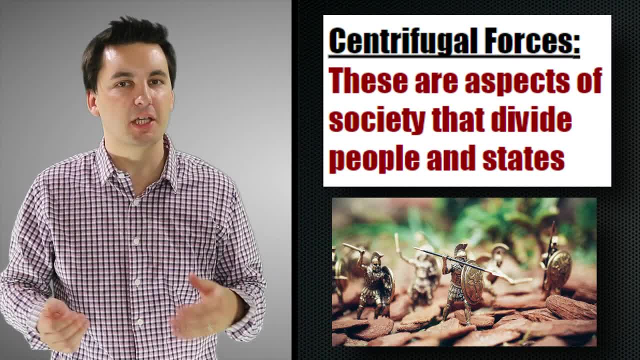 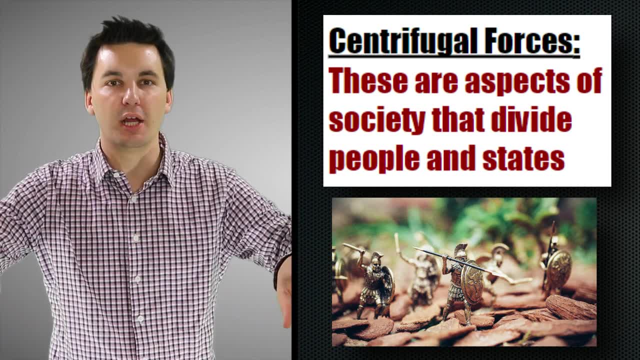 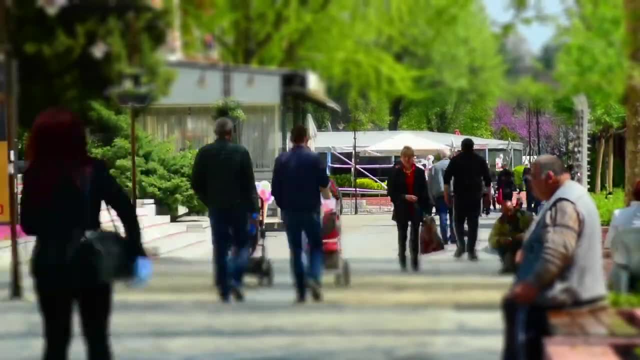 spoken, lack cohesion or have political and economic inequality or discrimination, will have centrifugal forces at play. these are forces that are pushing people apart. they actually cause the society to fall apart. they actually cause the society to fall apart and they pull people apart to crack, cause division within the community now, just because the society has multiple religions.